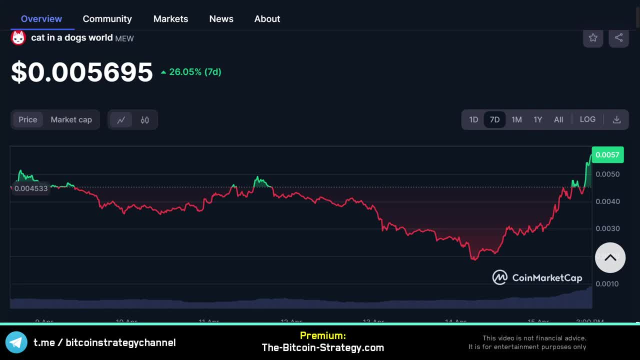 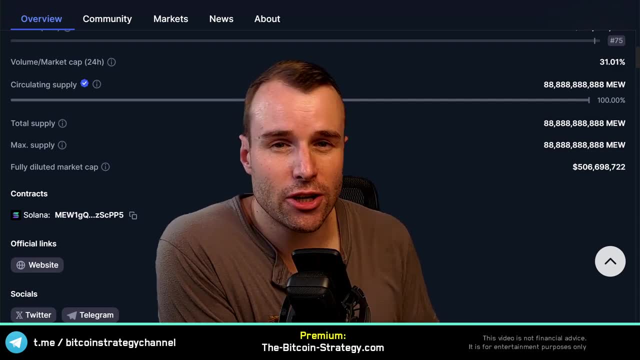 A lot of that decline was due to Solana itself going down. Here's the performance since listing on CoinMarketCap a clean 3x, And so all of the supply is currently circulating. The fully diluted market cap is roughly half a billion, And with that we still have quite a bit of upside potential. 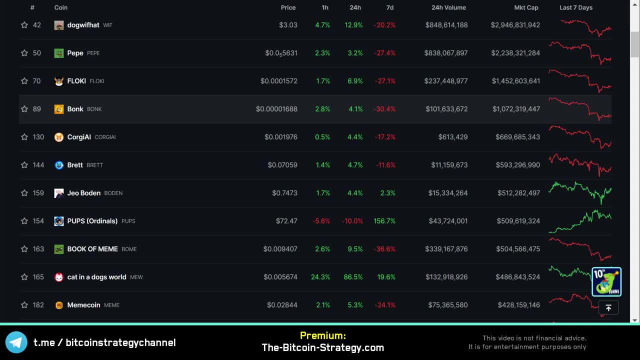 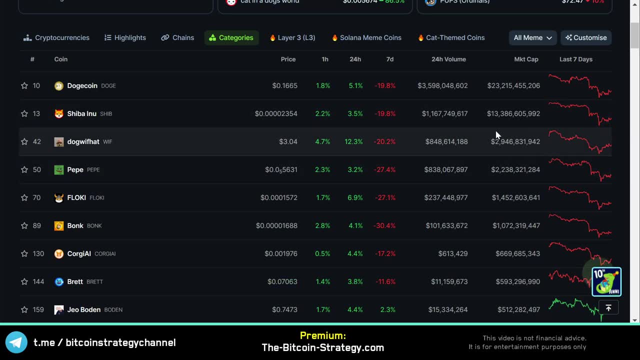 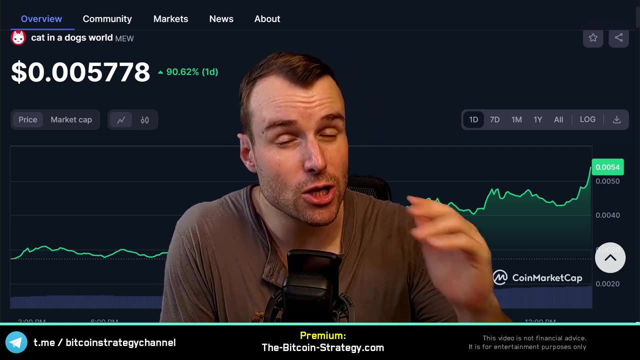 For example, Bonk is more than double the size, Floki Inu is triple the size, Pepe more than four times the size. The largest meme coin on Solana Dog with Hat is roughly six times the size. So if nothing else would happen in the world of crypto, the Mew token would be the largest of the 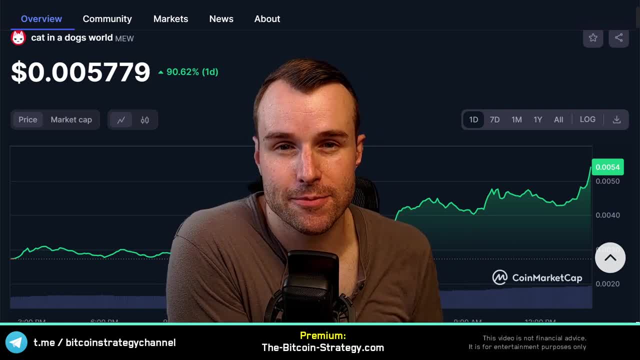 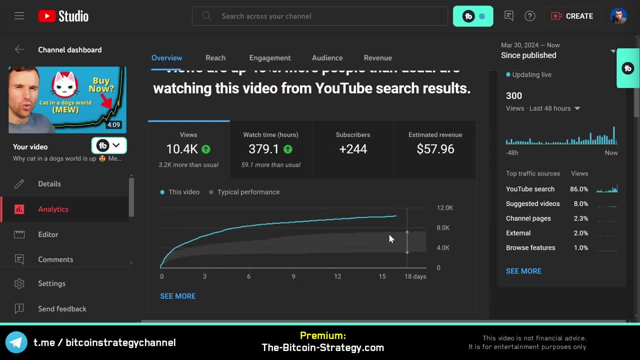 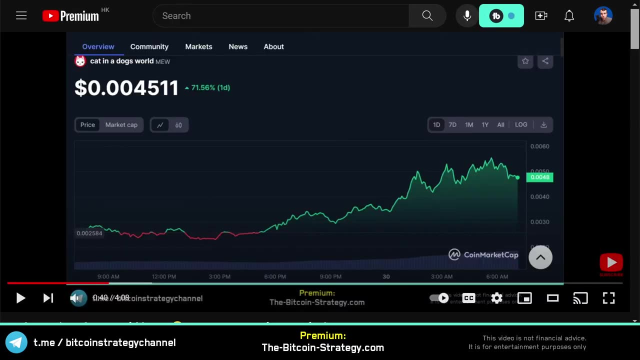 meme coins on the Solana chain at roughly three cents Now. two weeks ago I already published a video on Cat in a Dog's World. That video outperformed a typical video. The typical video here is in gray. Cat in a Dog's World got roughly double the amount of views At the time we were at 0.45 cents And again, Solana did not do too well during that time frame. So the Mew token really outperformed. because this is how meme coins in general are traded: They are traded on decentralized exchanges in a liquidity pool against a base token, And in this case the base token is SOL. 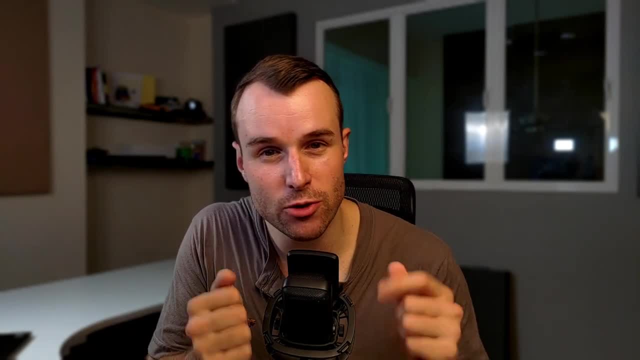 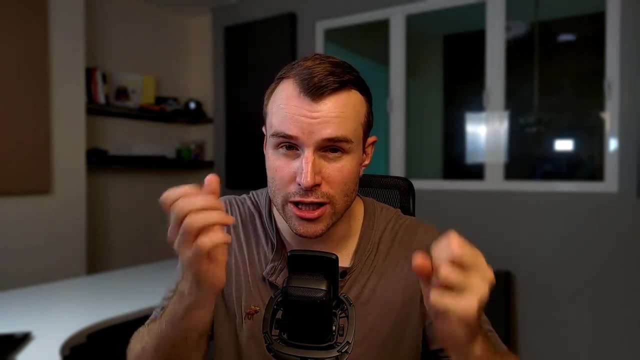 In other words, the price of an altcoin is not necessarily determined by the US dollar value. It's determined by the relationship in the liquidity pool between, in this case, SOL versus the altcoin. In other words, when SOL goes down by 10% or 20% in US dollars, then automatically. 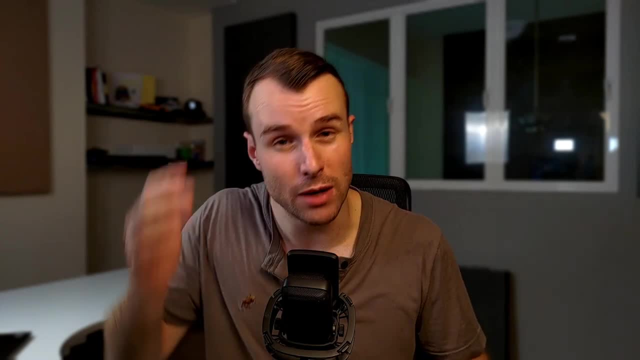 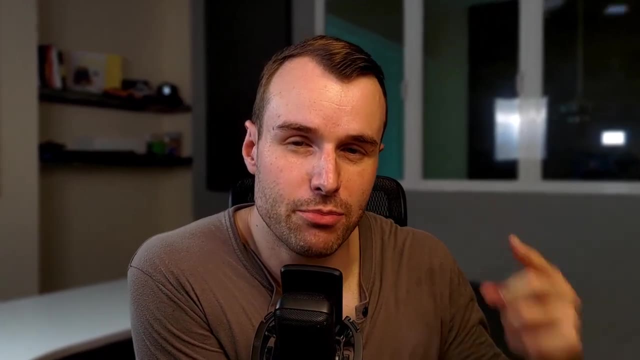 the US dollar price of the altcoin also goes down by 10% or 20%. There's a direct link here. Now let's have a look at on-chain data. Let's have a look at who's currently pushing up the price. 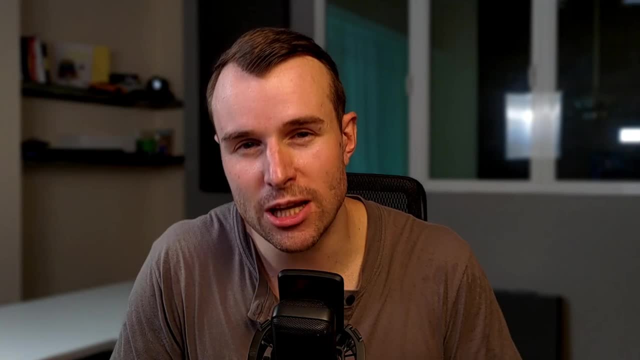 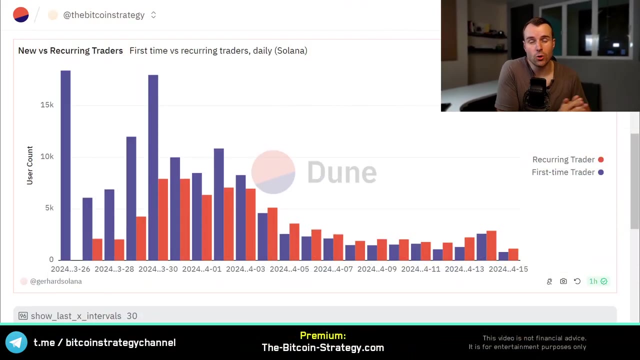 Is there a lot of new investors jumping on this or is there potentially some very large players that push this all up? Have a look at the following chart. I've built a tool for Solana tokens to look at the number of new traders versus recurring traders over time, So the Mew token was launched. 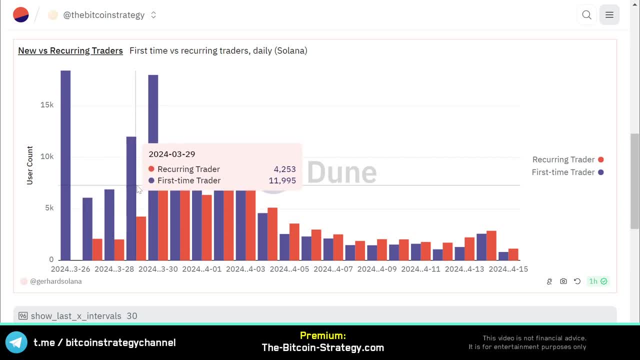 last year and is the number of new investors Now. this is right now in the US dollar. I think there is a lot of agreement here. All of the new investors that we've launched have some very large reason this time, before the 1st and 2nd and 3rd days of the 1st and 3rd days of the 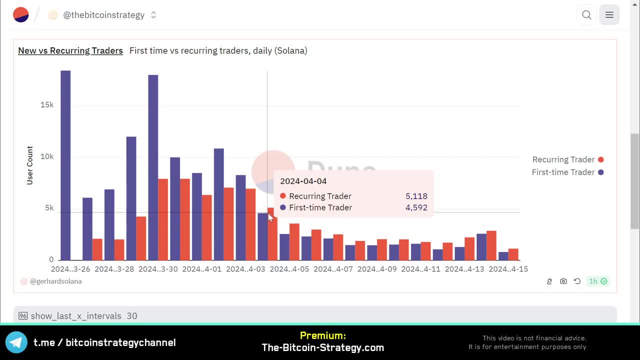 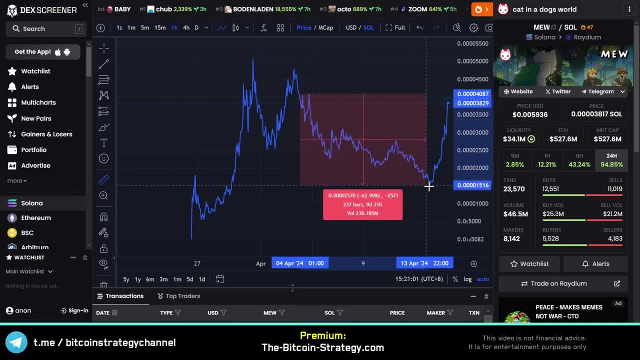 last year. The market is now pretty much up for the first time traders. Then for the subsequent days the number of first time traders exceeded the number of recurring traders. This is very positive because that shows us a growing investor base, more and more people getting onto a token. 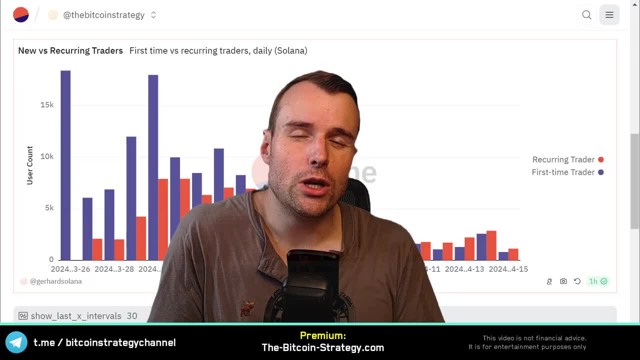 Means, of course, a rising price. But then on the fourth of April that has flipped and have a look even more, by roughly 70%. And so what do we learn from this chart here? We learn that the recent price rally is not organic. 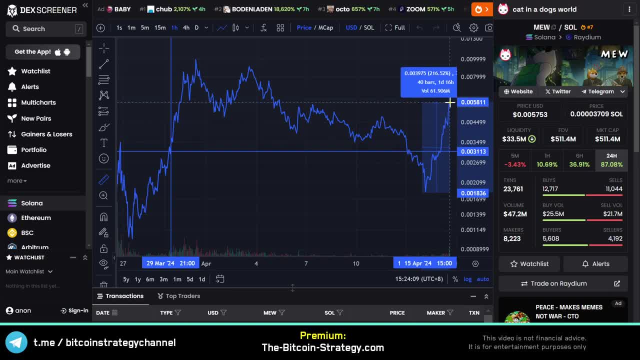 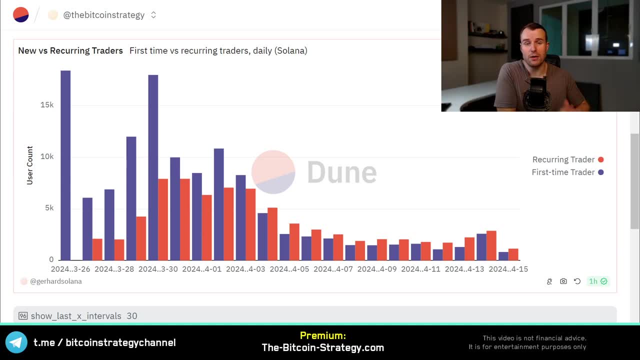 There's not a lot of new first-time traders here. The price is shooting up in SOL more than a 3X in just a few hours, but this is not due to broad adoption, due to a lot of people jumping on here. This is due to some very important people. 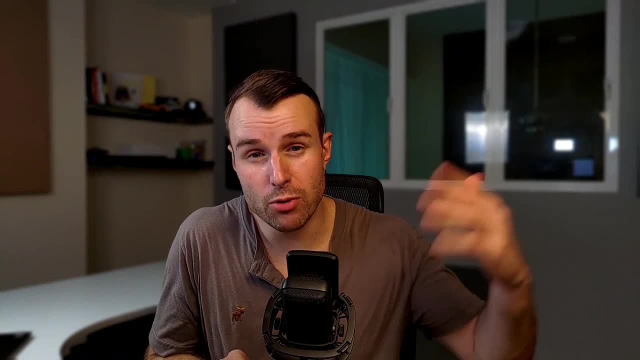 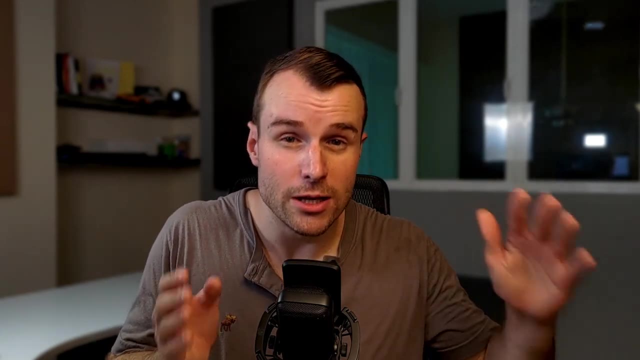 with very deep pockets getting in Now. how much longer will they push up the price? Your guess is as good as mine, but this is definitely not price action that will gradually slow down. This will very likely be very volatile, as in the price either shoots up further. 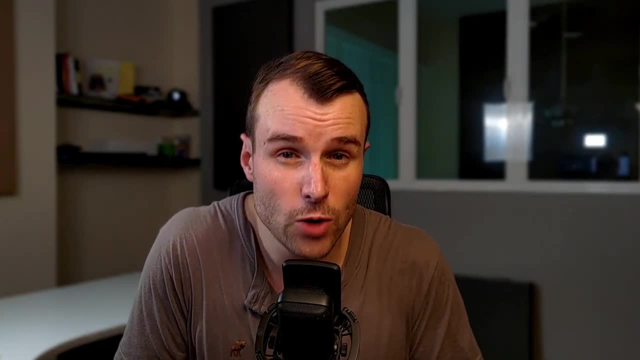 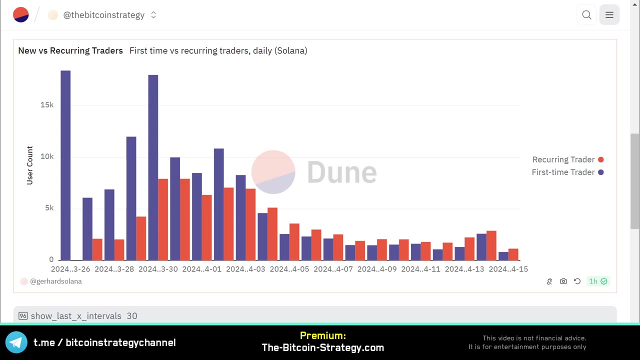 because it generates a lot of attention, or potentially it could also crash the price, in case people get on this with leverage, for example, on centralized exchanges like MACC. Now this tool- with this graph, by the way- is accessible for the premium members. 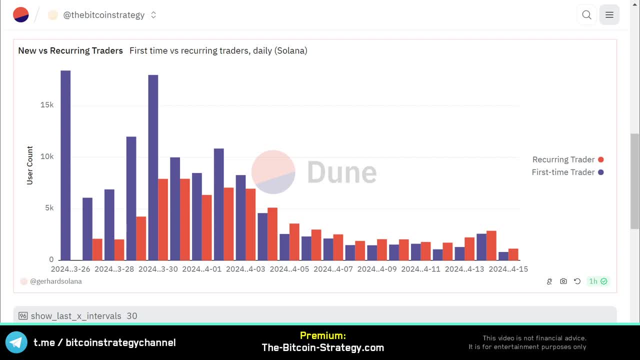 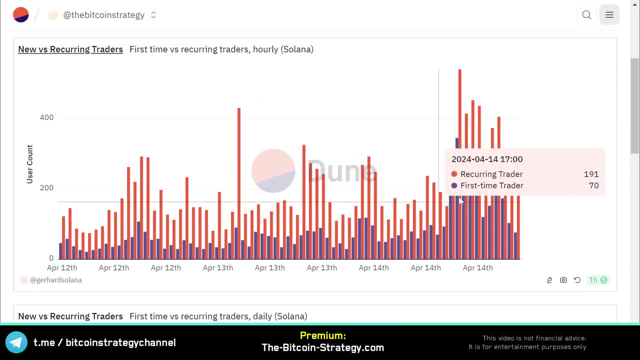 So feel free to check it out. thebitcoinsradiocom: You can plug in any Solana token in here to see the source of a potential rally. So I simply just entered the MUT token over here and we also get an hourly breakdown, by the way. 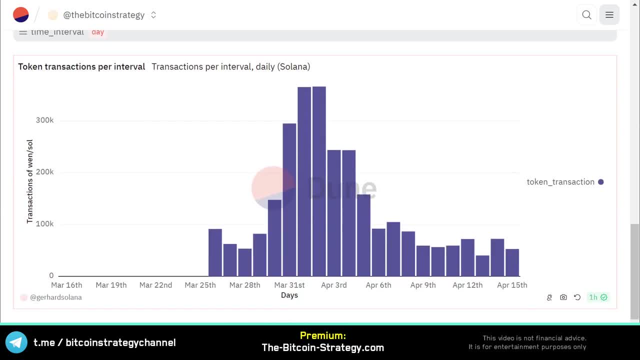 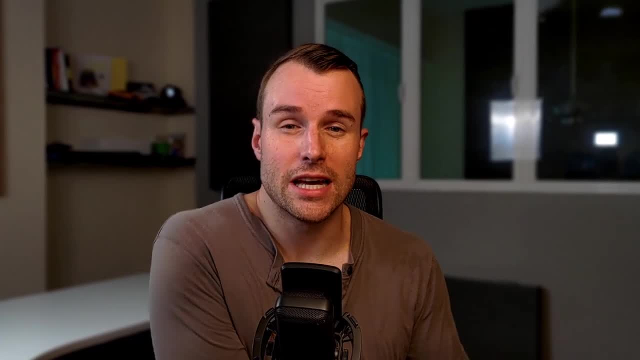 This is the daily breakdown, and here is the number of token transactions, Also not necessarily caused by a lot of new people entering here. Now, there is an effect that overshadows all of this, and that's, of course, the recent underperformance of Solana. 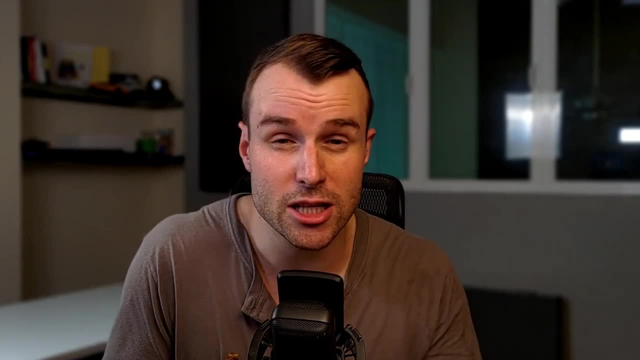 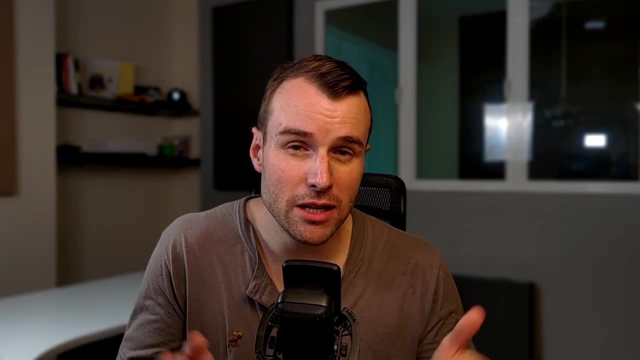 In general, the activity on the Solana blockchain is declining. I just published a video on SOL and on the activity of SOL on this channel yesterday. Feel free to check that out. But the main problem is simply valuation. It's a relative valuation to other cryptocurrencies. 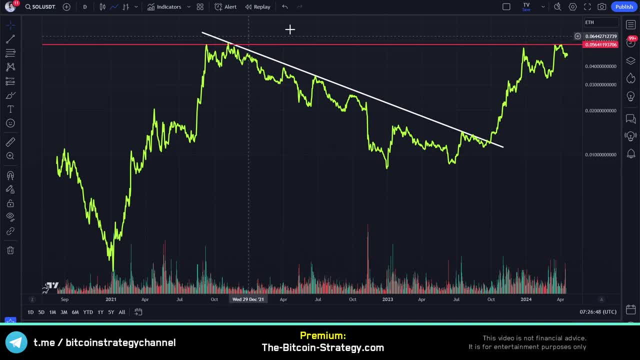 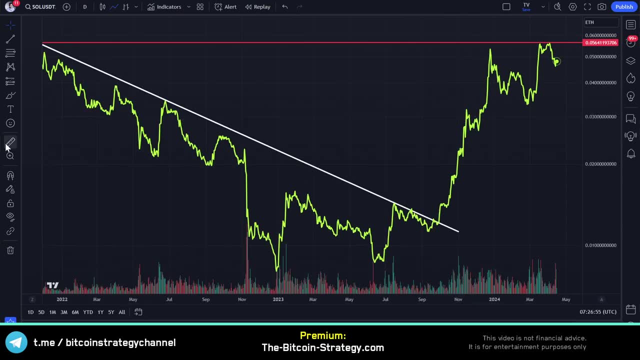 This here is SOL divided by Ethereum, and we are pretty much close to all-time highs, similar to what we had seen in November of 2021.. And the potential risk, just relative to Ethereum, compared to the reward, isn't that great. 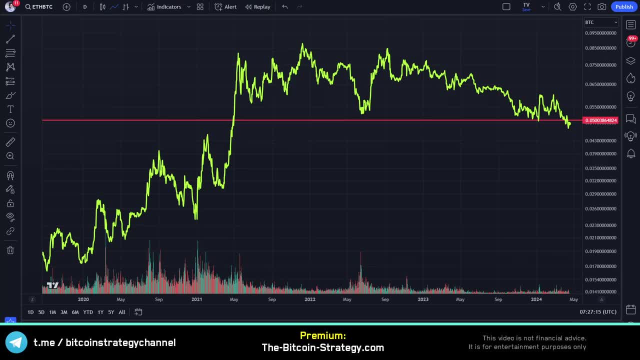 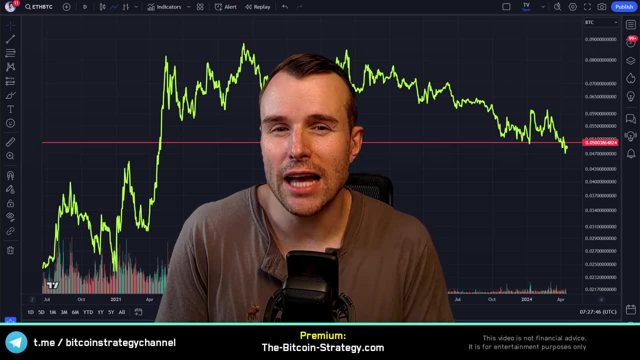 And that's again relative to Ethereum. Ethereum itself has a problem. This is Ethereum relative to Bitcoin. This is also pretty much bleeding since the change to proof of stake. So really, the climate is changing now. I believe that any altcoin speculation right now